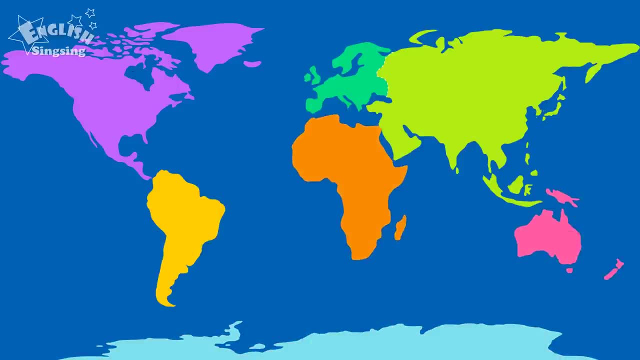 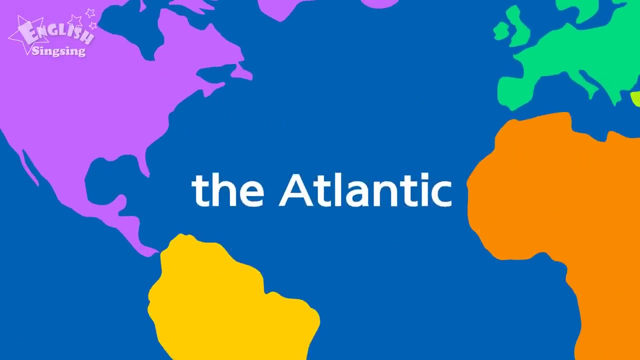 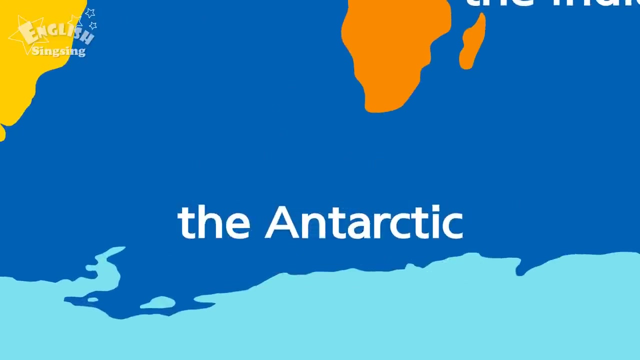 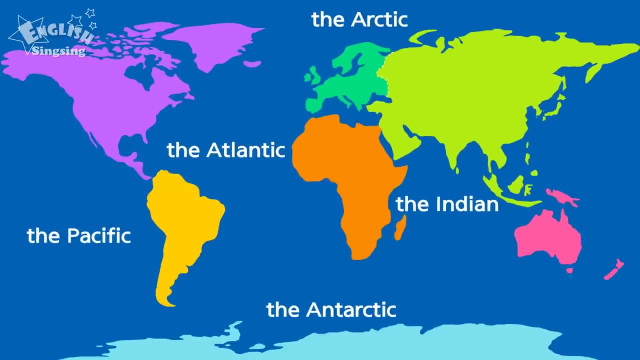 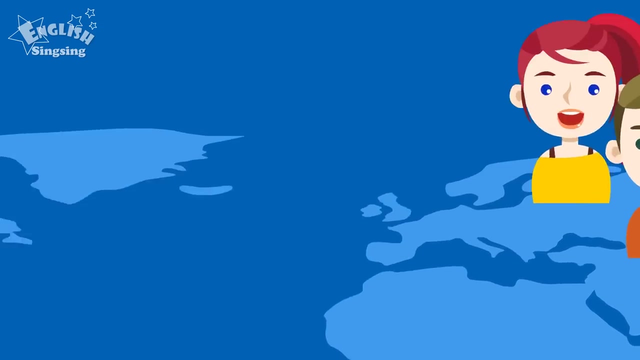 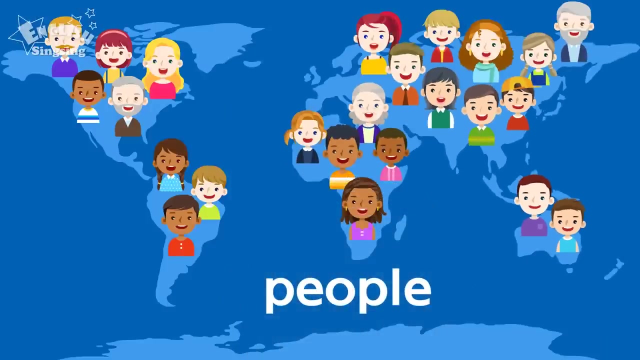 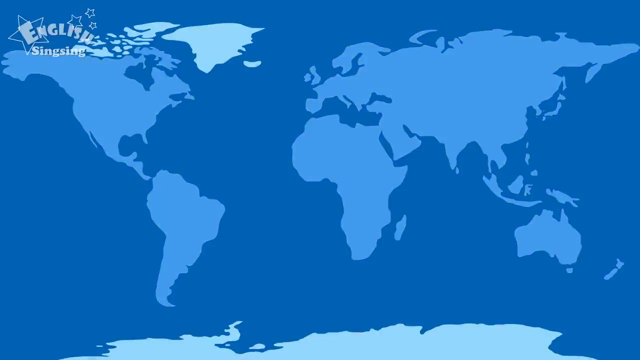 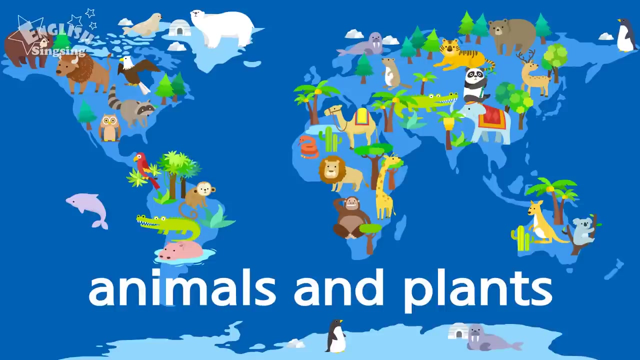 and Antarctica Oceans. There are oceans on the Earth Oceans: The Pacific, The Atlantic, The Indian, The Antarctic, The Arctic, The Pacific, The Atlantic, The Indian, The Antarctic and The Arctic Countries. There are about 200 countries on the Earth. Countries, people: there are over 7 billion people on the earth. people, animals and plants. there are various. 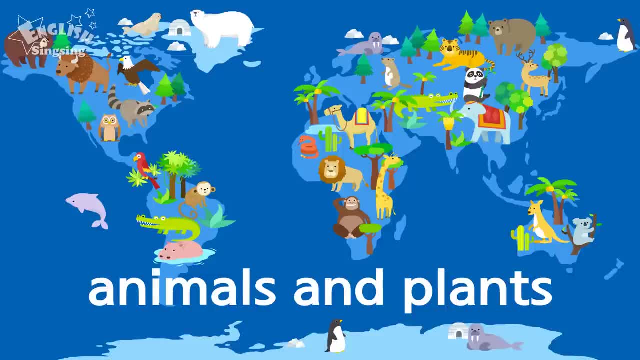 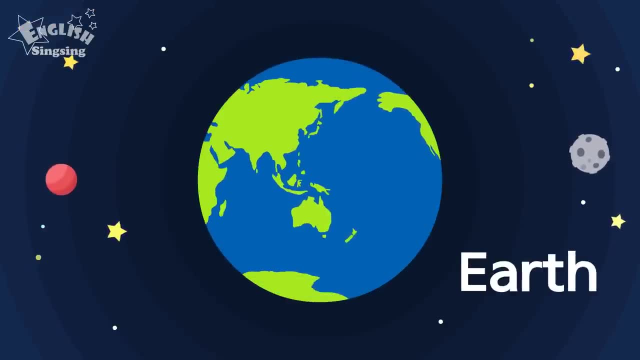 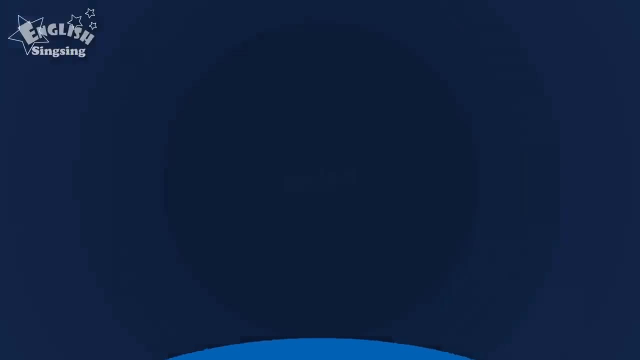 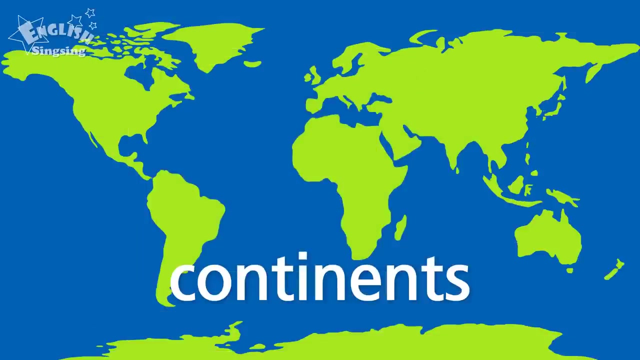 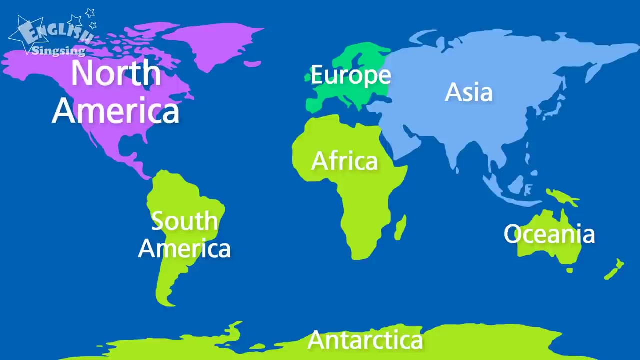 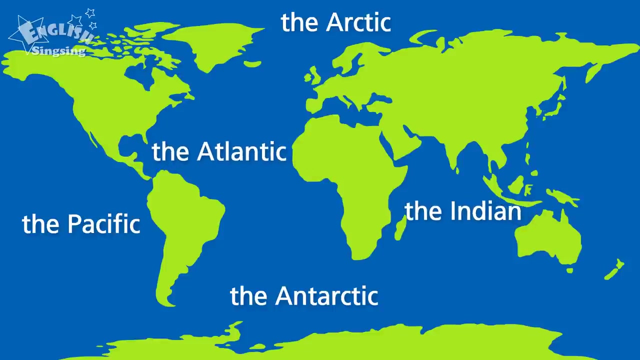 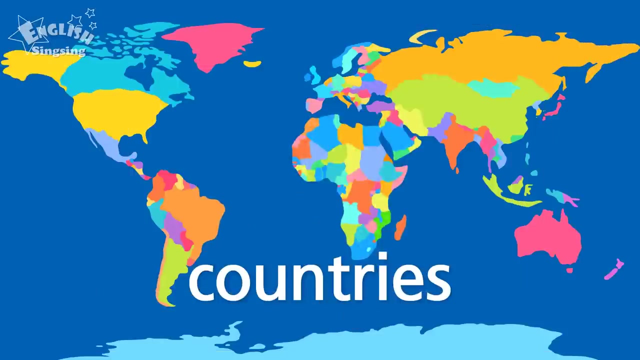 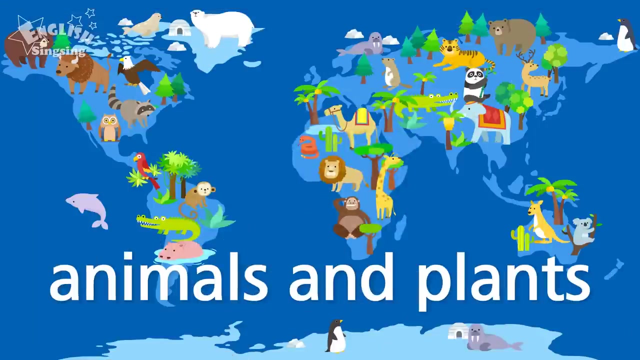 animals and plants on the earth. animals and plants, earth. this is our planet earth review. earth continents: Asia, Europe, North America, South America, Africa, Oceania, Antarctica, oceans, the Pacific, the Atlantic, the Indian, the Antarctic, the Arctic countries, countries, countries, people, animals and plants.